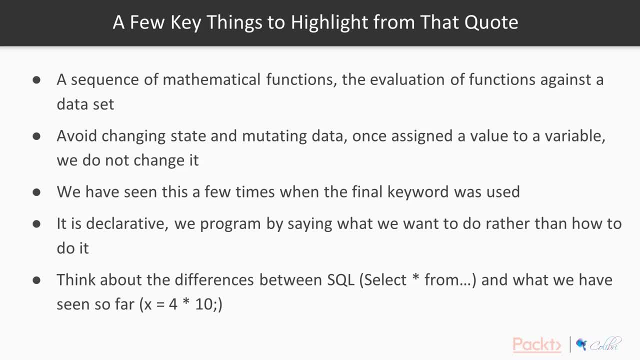 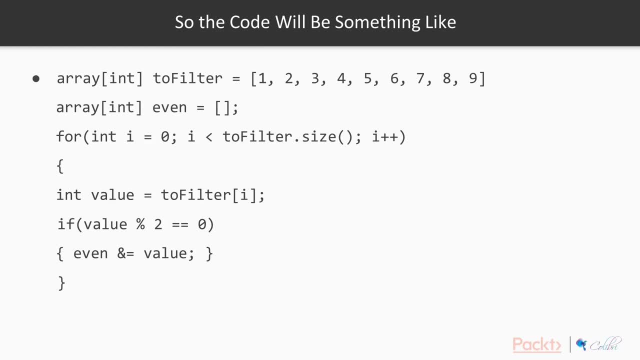 Next, evaluation of functions against a point in a dataset. and that's just put in place here and that's sort of the beauty of functional programming. all of this stuff is boilerplate. actually, the only piece of functionality that matters is our filter, because if we were going to apply a different filter to test if the number was greater, 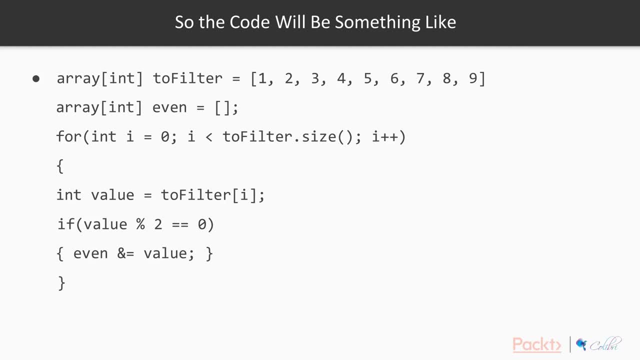 than five. all of this code would be exactly the same, except for this filter function here in the if condition. so essentially functional programming wraps all of that up for you and allows you to express it as a function that you want to apply to your list, and that's all this is. it's a function. 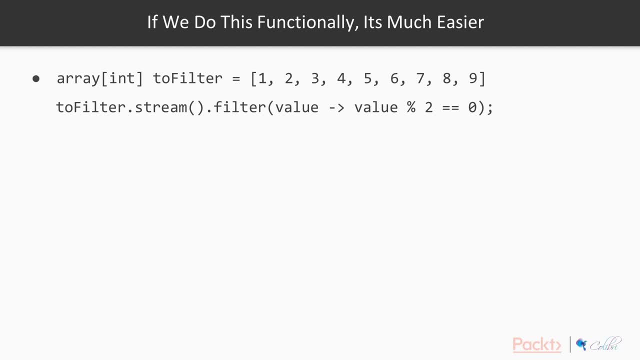 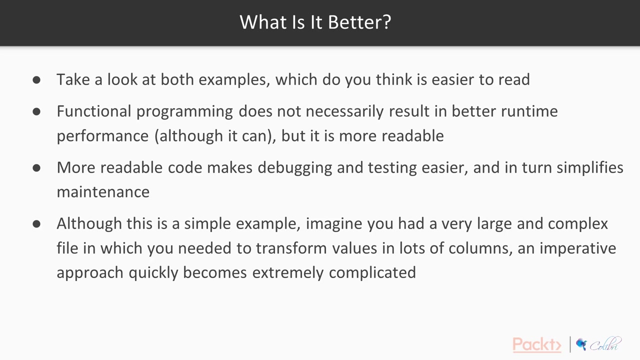 that we apply to our list of values. we want to apply a filter function, and this is the expression criteria. this is the evaluation criteria that gets applied against each element. so why is it better? well, take a look at both examples again. the imperative example is some eight or ten lines. 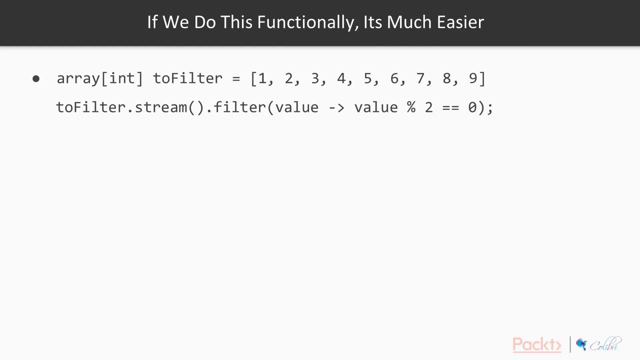 versus the functional example which, for intensive purposes, is one line which do you think is easier to read. if you saw this, you can see very quickly that we're applying a filter function to a list with this example. it's not obvious that it's a filter. you need to read through each line to understand what's going on and perhaps even debug. 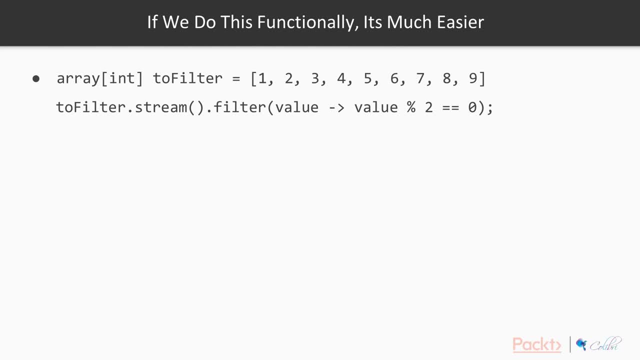 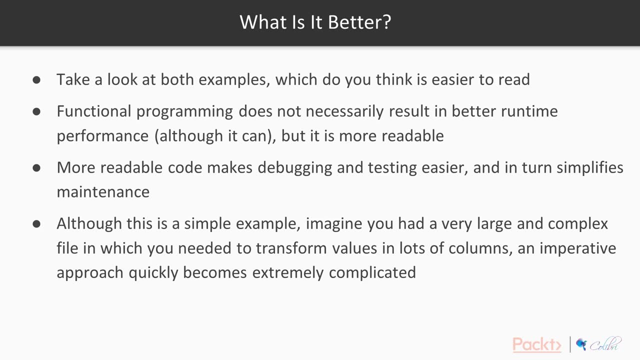 it yourself to figure out what's happening. this is very, very obvious. what's going on? functional programming doesn't necessarily result in better runtime performance, although it can under the hood. the compiler still has to do the same thing and the jvm still has to execute essentially the 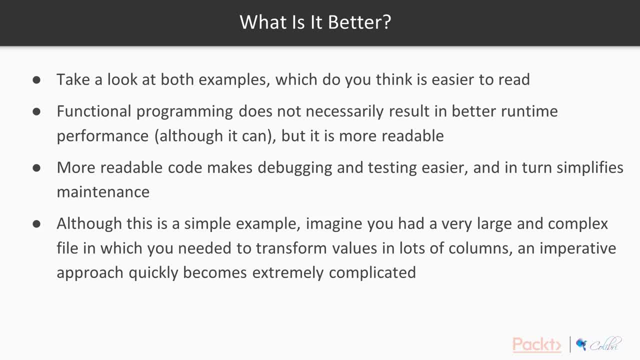 same stuff, but what we get to write is so much more readable and so much faster to write and therefore much easier to debug, much easier to test and, of course, in turn, much easier to maintain. because it's so much simpler, it's less easy to make mistakes. there's not a lot of room for mistakes. 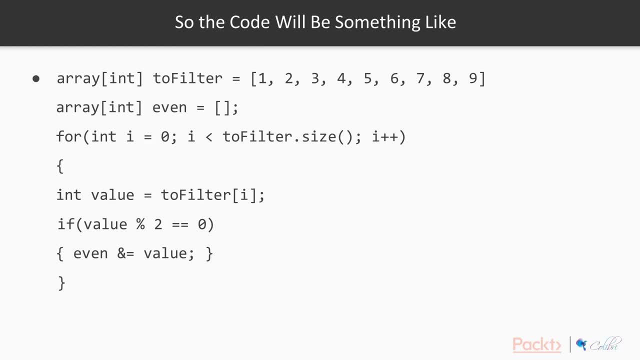 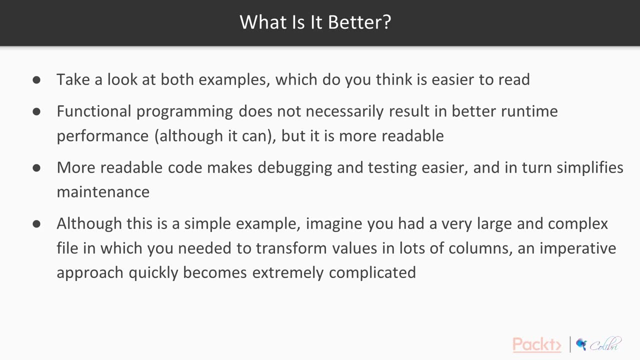 in this code, whereas in this it will be very easy to make a simple mistake and the whole function will be fail. Although this is a really simple example, imagine you had a very large and complex file that you wanted to transform. Perhaps you have many, many columns in that file and you want to transform it. you want 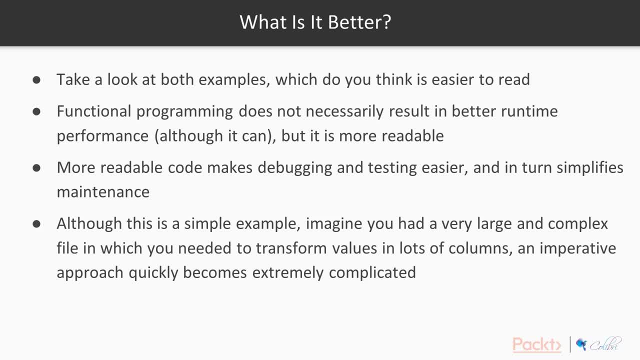 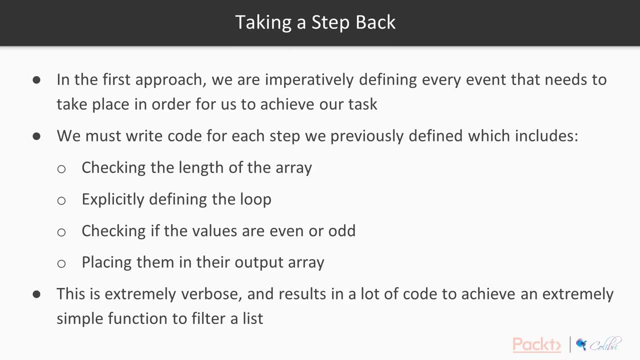 to filter it. you want to do some slicing and dicing of the data. An imperative approach quickly becomes very, very complicated, whereas a functional approach does not. So let's just take a step back for a second. In the first approach, we're imperatively defining every event that needs to take place. 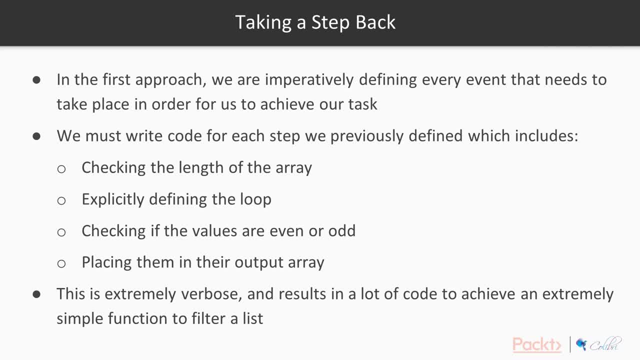 in order for us to achieve our task. So we go through and we write an exhaustive list of computational steps that need to happen in order to perform the task that we want. We have to write code for each step we previously defined from checking the length of the array. 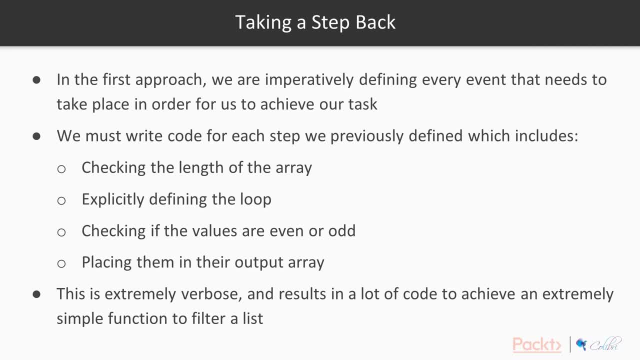 to explicitly defining the loop all the way through to checking if the values are even or odd and then placing them in their output array. This is really, really verbose and, as we've seen, it results in a lot of code to achieve. 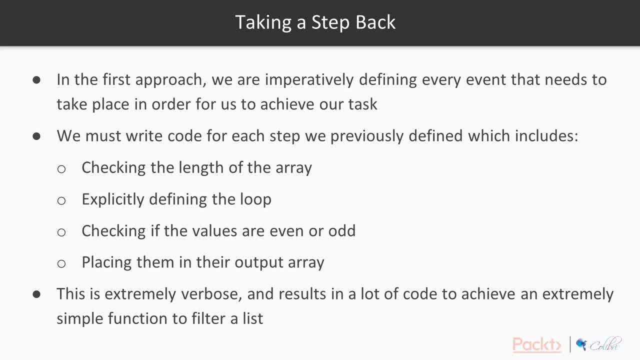 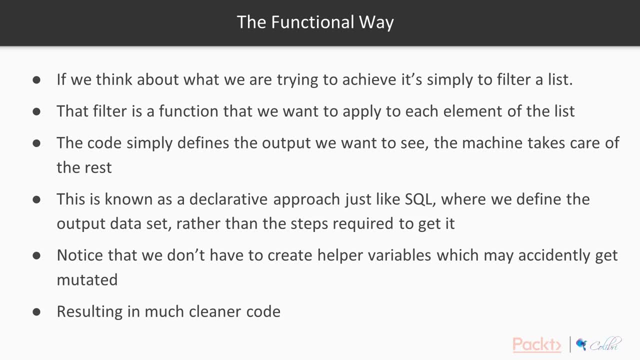 an extremely simple function, which is just to filter a list of values. Now, thinking about this, the functional way, if we think about what we're trying to achieve, it's really simple actually. We just want to filter a list. We don't care about iterating over every element, we don't care about all the other stuff that 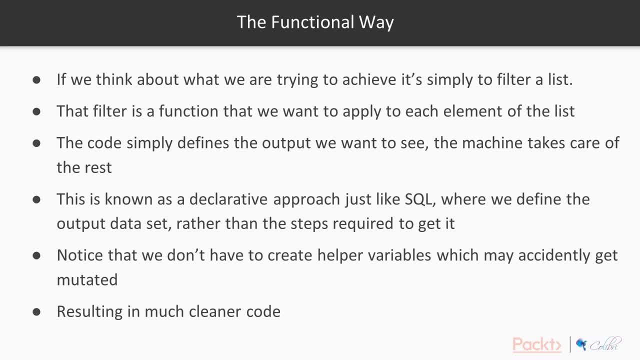 goes on. All we want to do is filter a list, and that filter is a function that we want to apply to each element. We can do this by defining a list. we don't want to use this thing. we want to define only the output. so we need to define a list which does what it wants, and that list should. 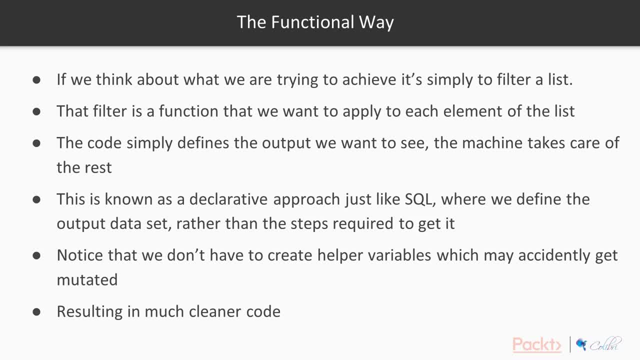 be the number of elements that are going to be there in this list. So the code simply defines the output we want to see and the machine takes care of the rest, as opposed to writing a list of instructions the machine must take or the computer must. 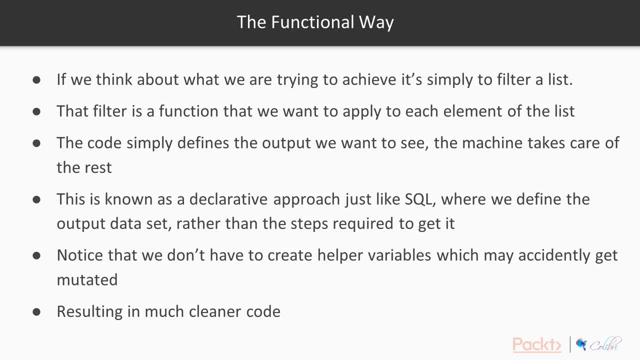 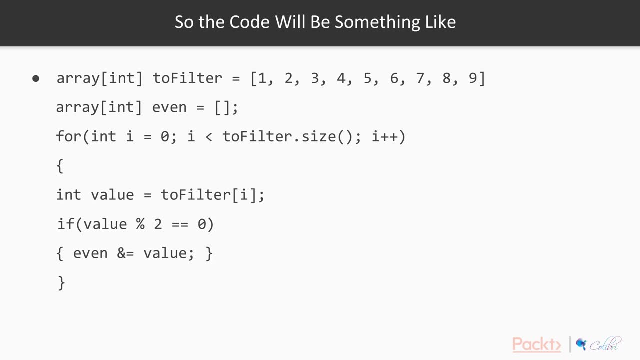 take. what we're doing is defining declaratively what we want the output to be, So this is known as a declarative approach. just like with SQL, where we define the output accidentally get mutated. so in the previous example we essentially created a helper variable, here an even array which we're mutating. so this is exactly. 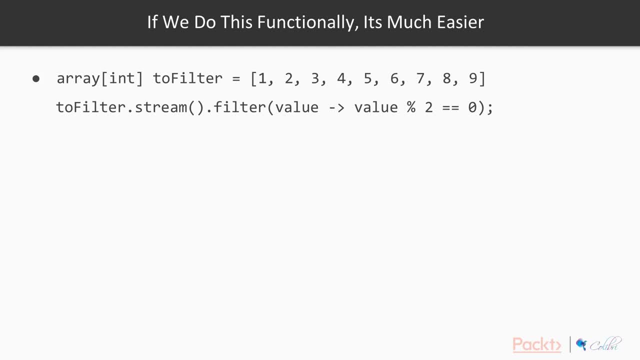 what I said previously we would try and avoid, whereas here there's no mutation of data, there's no filter, there's no updating of arrays. all we do is we filter our list, so this doesn't get mutated at all. this stays the same. if we want to retrieve the value of this, we just collect it into a new list and of. 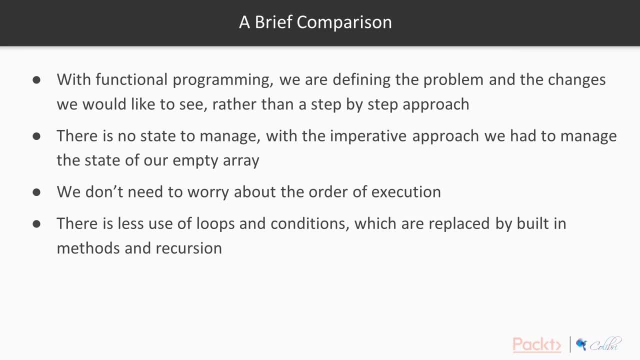 course, the result of this is much, much cleaner code. so a little comparison with functional programming. we're defining the problem and the changes we'd like to see, rather than an explicit, imperative, step-by-step approach. now there's no state to manage, there's no array of even numbers that we have to mutate, no state. 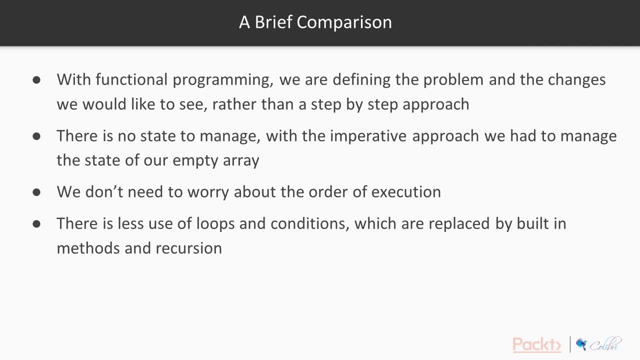 at all with the imperative approach. remember, we had to manage the state of our empty array. we had to make sure it started off as empty. we had to append values to it. we had to make sure it started off as empty. we had to make sure it was of the right type. with functional programming we don't have to do this and 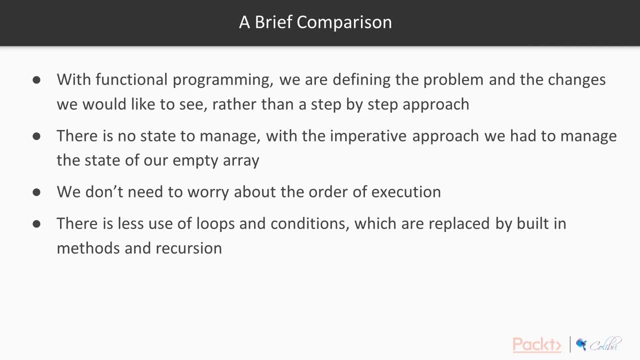 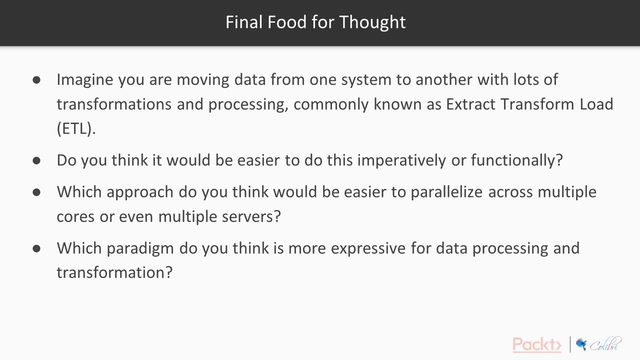 we don't need to worry about the order of execution either either. there's less use of loops in general and conditions, and these are replaced by built-in methods like filter- that we've seen- and recursion. so a last little bit of food for thought for this video and then we'll wrap up. imagine you're moving data. 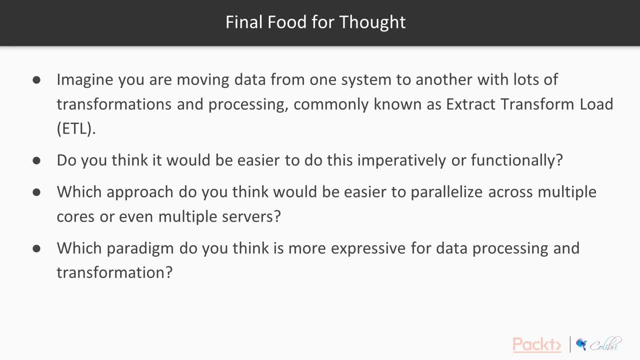 from one system to another with lots of transformations and lots of processing is commonly known as an ETL or extraneous. so we can use the data warehouse to extract, transform and load process. so say, we've got. we've got an application database and a data warehouse we want to 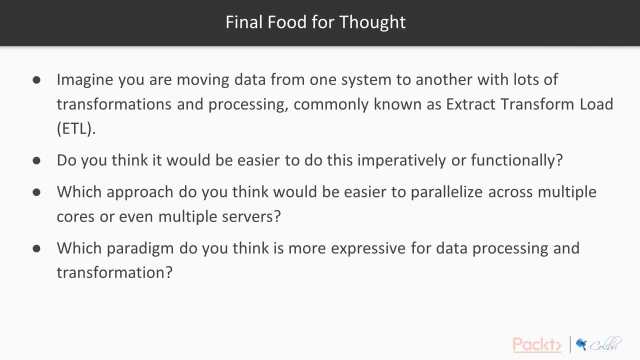 move data from our application DB into our data warehouse. we're going to build something called an ETL pipeline and it's going to extract data from the source system, do some transformations and processing on it, maybe some filters, and write the output into our data warehouse. do you think it would be easier? 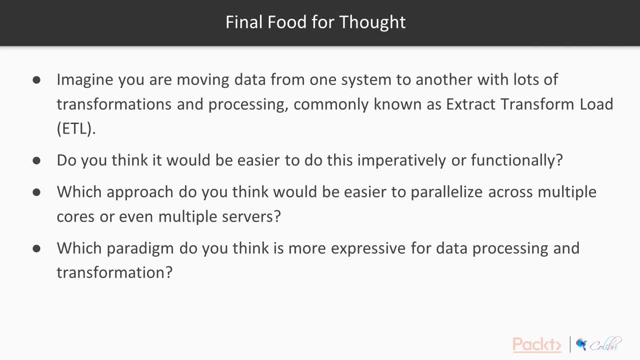 to do this imperatively, using loops and lots of conditions and state variables, or functionally? and which approach do you think would be easier to parallelize across multiple cores or perhaps even multiple servers? which paradigm do you think is more expressive for data processing and transformation? now I'm going to leave those thoughts with you.